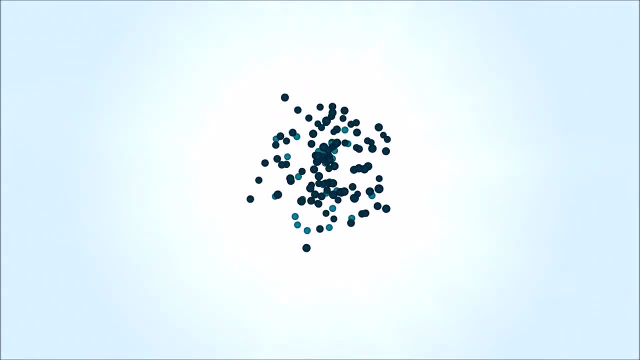 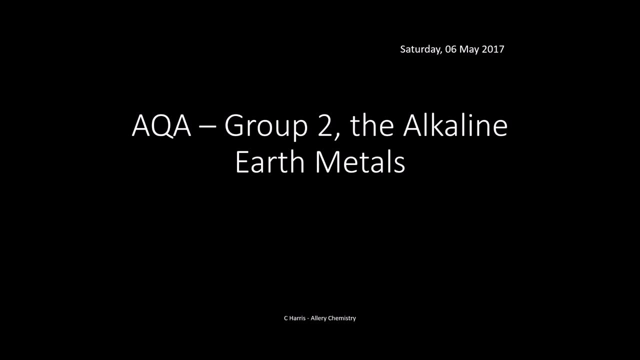 Hello and welcome to this video. This is the AQBA, Group 2, the Alkaline Earth Metals. My name is Chris Harris and I'm from AlleryTutorscom and in this video we're basically just going to go through just an overview, really, of the Group 2 topic, So it's like a revision video. 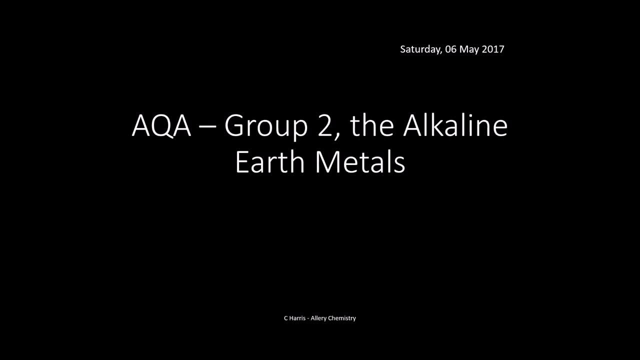 effectively. Just a quick thing to say as well that I'm going to use this PowerPoint that I've made. Now, if you want a copy of this PowerPoint, or if you need, if you'd like to print it off and use it for revision, etc. it can be purchased from the link in the descriptions. 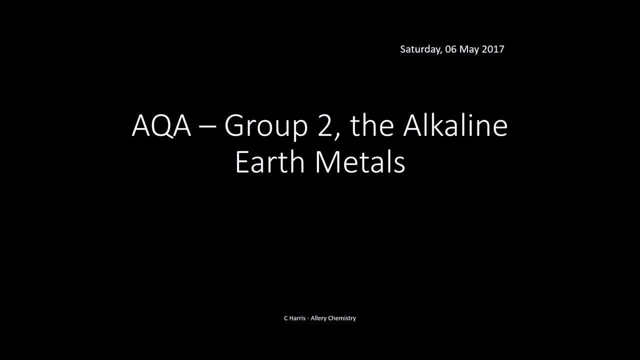 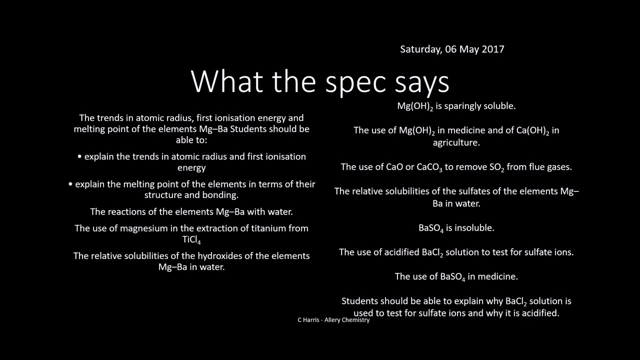 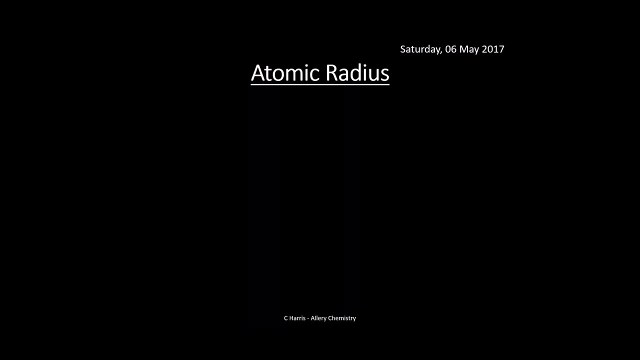 box underneath this video, So if you just click on the link, you'll be able to get a hold of it there. Like I say, this video is very specific to the specification. This is the points from the AQA Group 2. So everything on here should be relevant if you are studying the AQA syllabus. 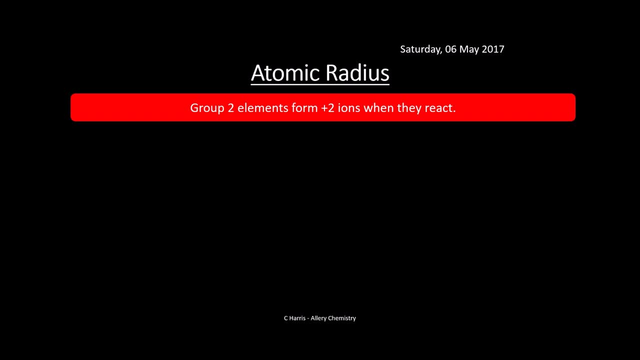 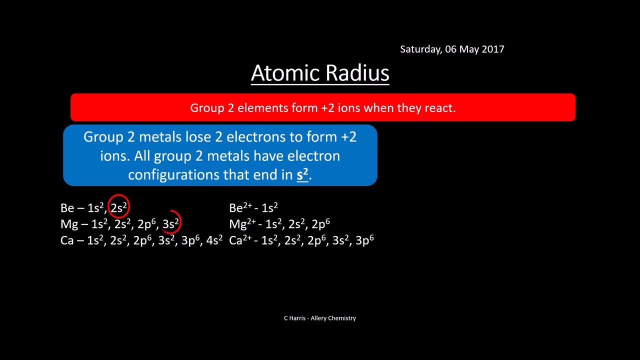 Okay, so let's start with atomic radius. So basically, Group 2 elements form plus 2 ions when they react. So basically they're all Group 2 metals and they always have this configuration that ends in S2.. So you might see them here. So you'll see that Beryllium ends in S2, Magnesium. 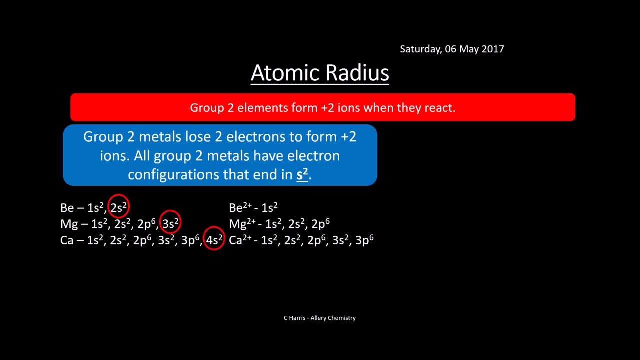 ends in S2 and so does Calcium, And basically, when we lose 2 electrons from these elements, we form the 2 plus ions, as shown here, And these are the electron configurations there. So the atomic radius as we go down the group increases. So that's pretty important because 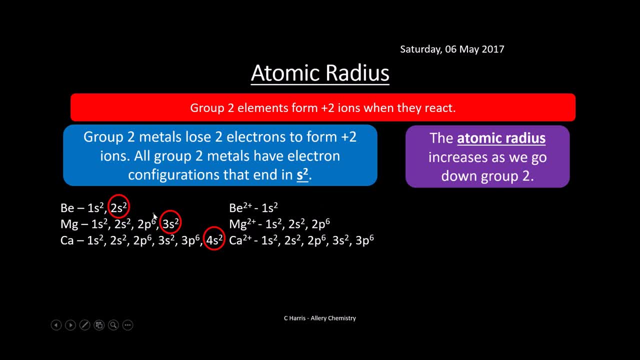 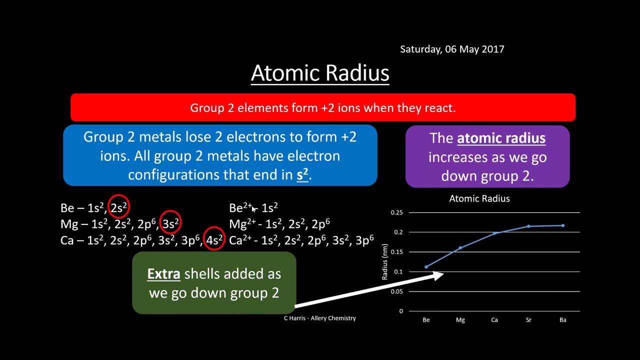 we're obviously adding extra electron shells here, you can see. So it's getting bigger and bigger as we go down the group, And there's just a graph just to prove that. So extra shells added as we go down the group. Okay, ionisation energy. 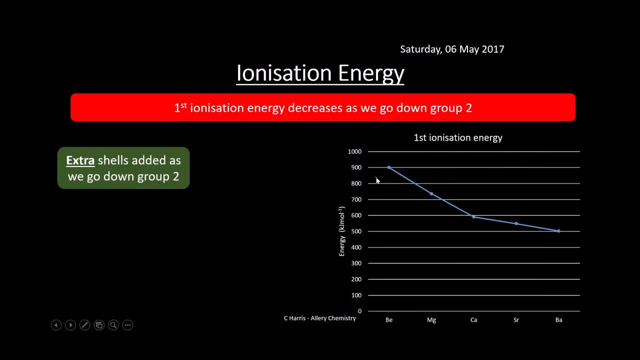 Decreases as we go down the group. This is because- and here's the graph here- This is because we add extra shells as we go down the group, as we'd seen just earlier, And this basically leads to shielding, And we're using this word again: shielding. So there's more. 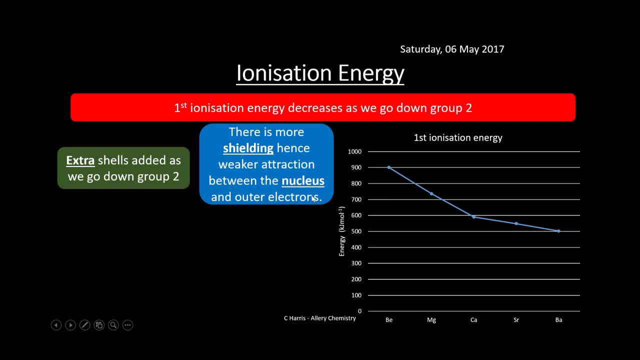 shielding. hence we get a weaker attraction between the nucleus and the outer electrons. So as we go down- obviously down Group 2, the first ionisation energy gets lower. because of this shielding, The outer electrons are further from the nucleus and this weakens. 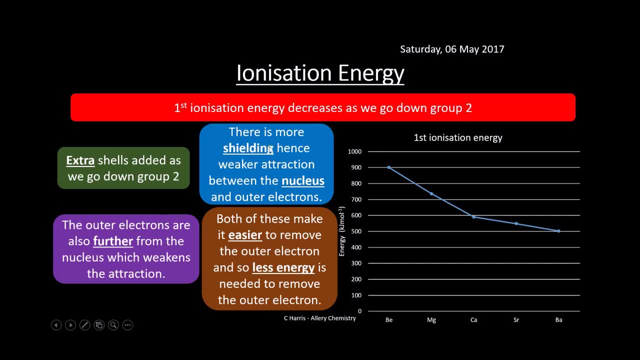 the attraction And basically both of these effects make it easier to remove that electron from the outer shell. as we go down the group, Less energy is needed. So really important there using the word shielding, and further from the nucleus etc. So bigger atom etc. 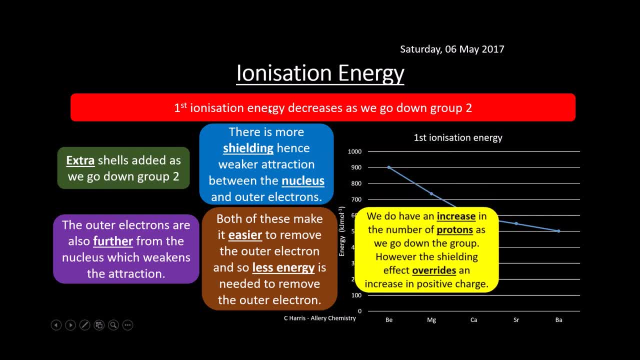 as we go down the group. Really important there, Okay. so it's also important to note, I suppose, that as we go down the group, we do get an increase in the number of protons. However, the shielding effect overrides this increased positive charge in the nucleus, So it's just. 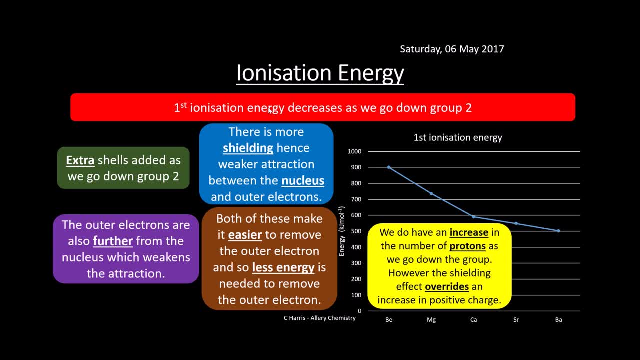 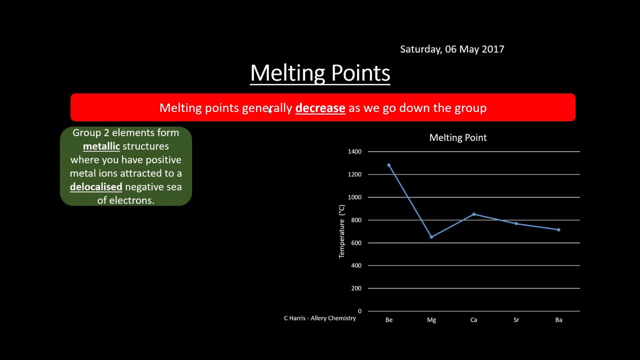 worth noting that, because they might ask a question on that. but shielding always overrides it. Okay, melting points. So melting points generally decrease as we go down the group. So you can see here the main reason is because we've got this. obviously we know that metals are. 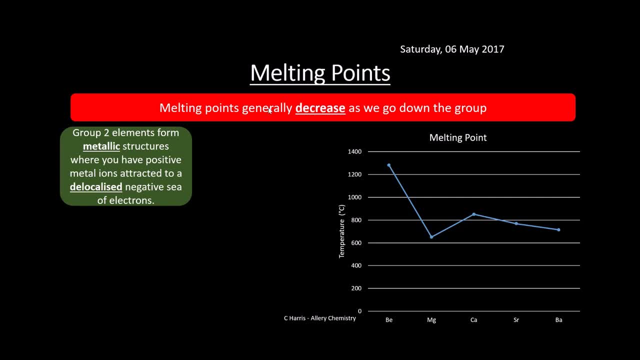 that Group 2 are metals, so they have metallic bonding And metallic bonding is basically where you have a positive metal ion and delocalized electrons or negative C of electrons. Now as we go down the group, the size of this metal ion increases, But the number of delocalized 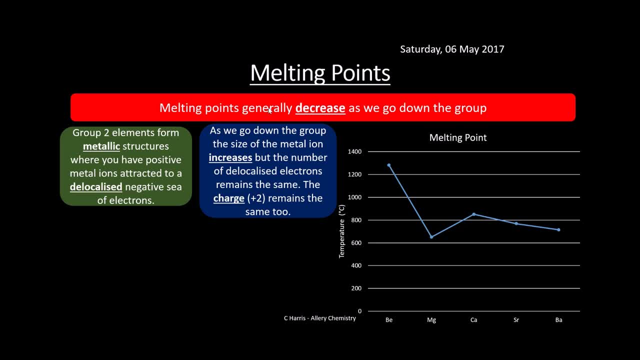 electrons remains the same, And so does the charge on the metal ion as well. that remains the same, And basically this means that because the ion gets bigger but the charge and the number of electrons remain the same, Then the distance between the delocalized electrons and the hot 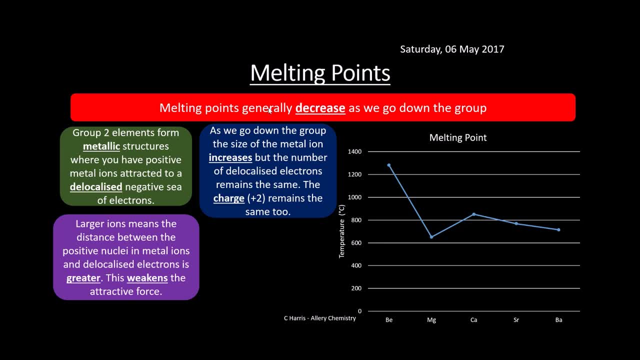 electrons in the nucleus and the positive metal ion gets bigger, and so because that gets bigger, that weakens the attractive force and this means it makes it easier to effectively break these bonds and therefore the melting point is lower. and you can see, here we've got this general decrease from 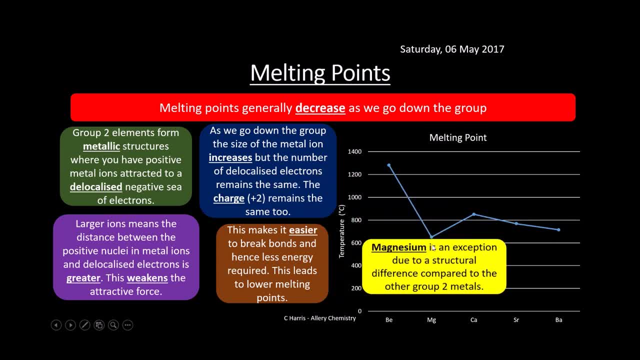 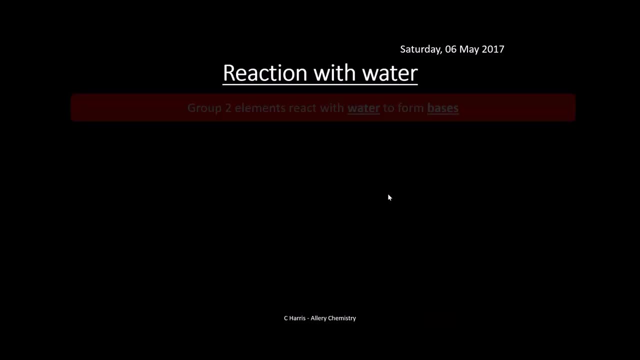 beryllium to barium. Now there is this exception which is magnesium, but this is due to some structural arrangement of magnesium and effectively this just gives it this exception. You don't need to know much about that, really Okay. reactions with water is obviously really important. They react with water and they 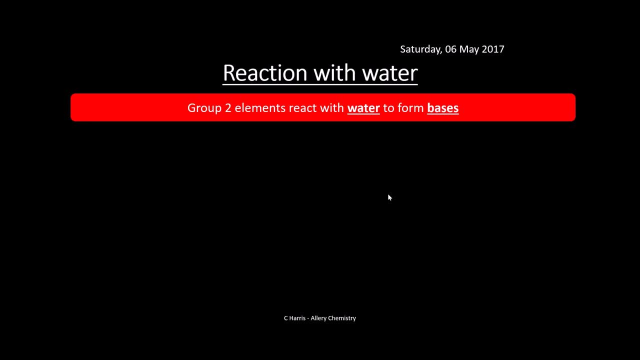 form bases. Now the whole point of this topic. this topic is called group 2, alkaline earth metals, and that's because when we react them with water, they form alkaline substances. So let's have a look. So these react with water to form metal. 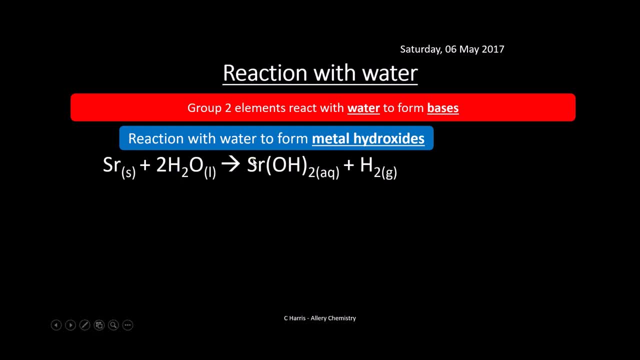 hydroxide. So here's an example. This is strontium reacting with water to form your hydroxide and hydrogen, Very similar to the reactions of group 1 metals. except group 1 metals are much more reactive than group 2 with water, but they still form hydroxide. Another thing to point out: 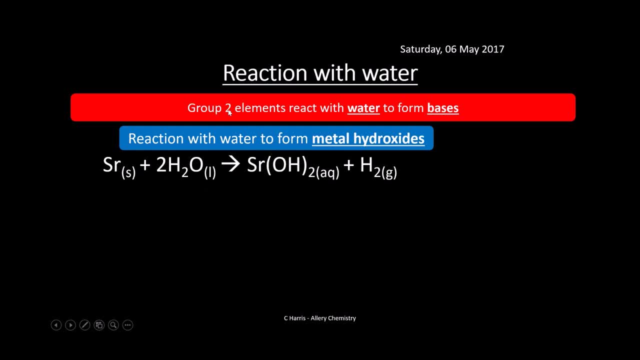 here is: if you look here, strontium is in group 2, all these, obviously all these group 2 elements. they form hydroxides, but make sure that you have two hydroxides bonded per group 2 metal atom and it makes sure it's balanced, That's. 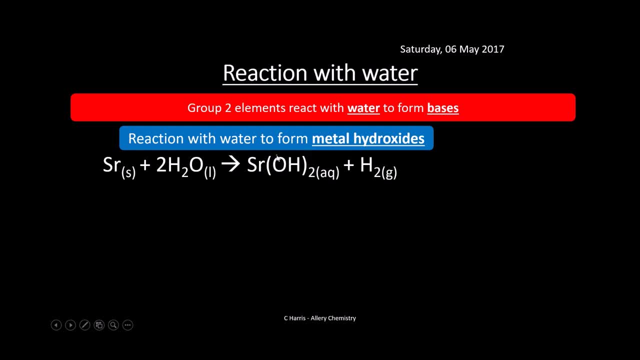 quite important. Some people just put OH and forget to put the bracket and the 2 there. So, yeah, OH is minus, strontium is 2 plus. you need two of them. So that's the way it works To balance that out, and hydrogen gas is obviously produced as well. 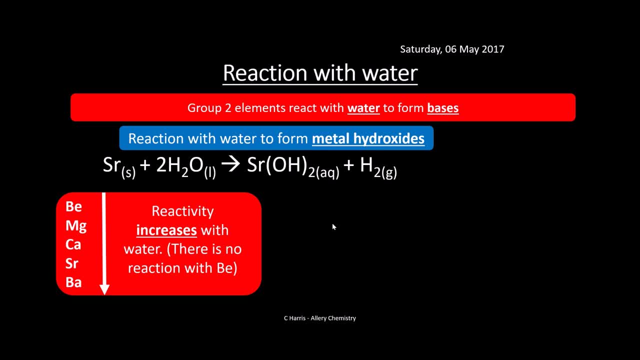 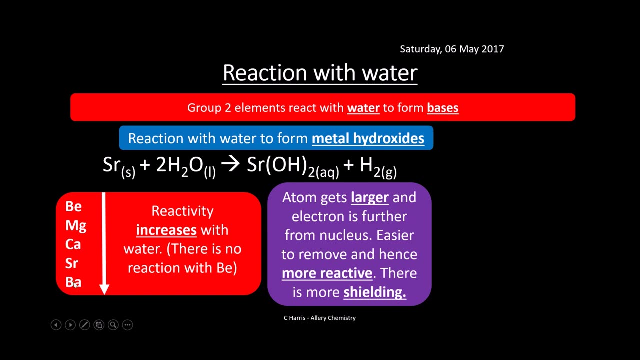 Okay, reactivity increases as we go down the group and, just like with group 1, metals and no reaction with beryllium, though, it's pretty unreactive, so it doesn't react with water and and the reason why is the atom gets larger as we go down the group, The electrons further away from the nucleus. 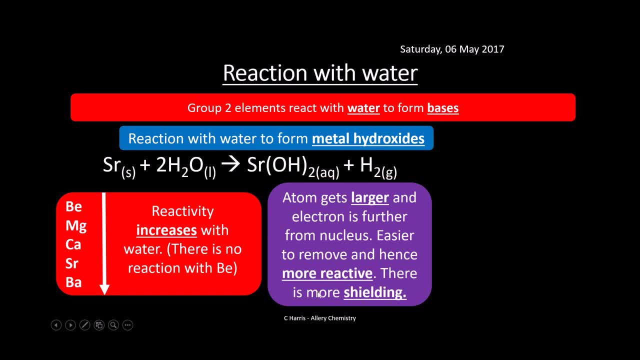 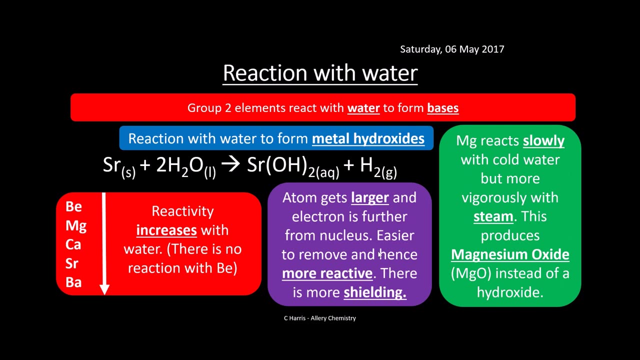 as we go down. So that means it's easier to remove that electron, more reactive, more shielding as we go down the group, and so that makes the, the metal, more reactive. There's a little bit of an exception though. Magnesium reacts slowly with cold water. okay, but it's a lot more lively when you react to the. 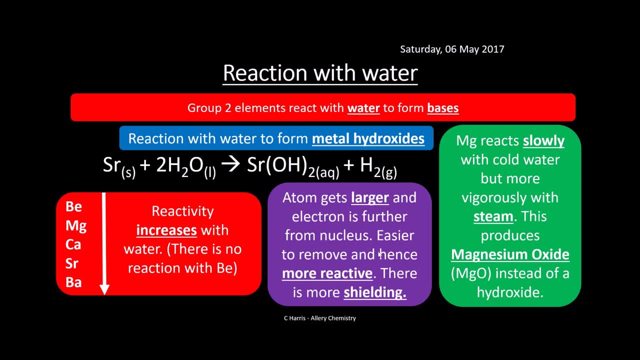 steam. so it's obviously it's a higher temperature. but another weird thing is that actually, when we react to magnesium with steam, we don't produce a hydroxide, we actually produce an oxide. we produce magnesium oxide. So just watch out for that one there and make sure that if they're talking about magnesium, 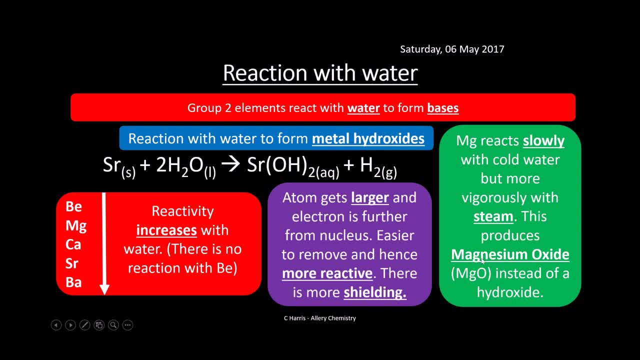 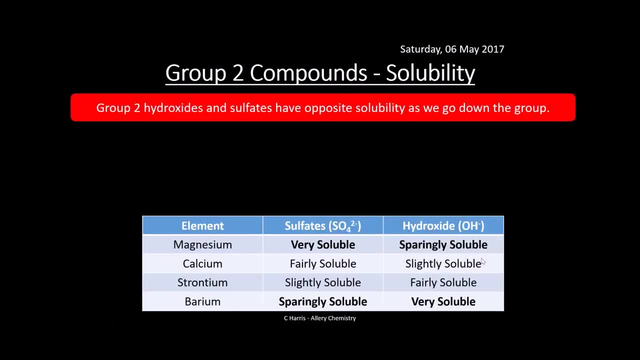 and steam that you actually produce an oxide and not hydroxide. Okay, solubility: obviously this is quite important because we're talking about how soluble these things are. So group 2 hydroxides and sulfates have opposite solubility as we go down the group. So, as a general rule, 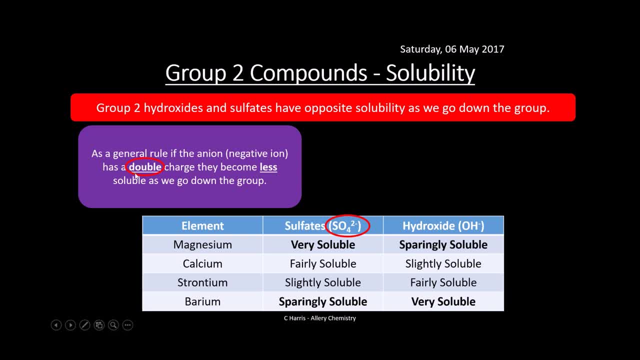 if the anion, the negative ion, has a double charge, they become less soluble as we go down the group. In other words, they become more insoluble. so you can see here, magnesium sulfate is very soluble because that's at the top the group. but as we go down the group to barium, barium sulfate is very, very well, it's pretty much. 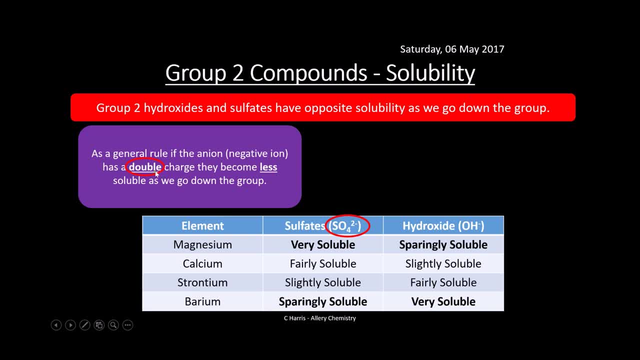 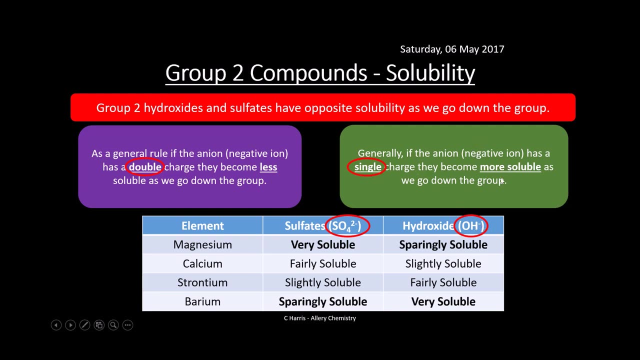 insoluble. it doesn't really dissolve whatsoever. so, um, this, basically, because this is a double charged anion, so42 minus, it becomes less soluble. if we look at the hydroxide, though, generally, um, if it has a single charge, like a hydroxide, they become more soluble as we go down the group and 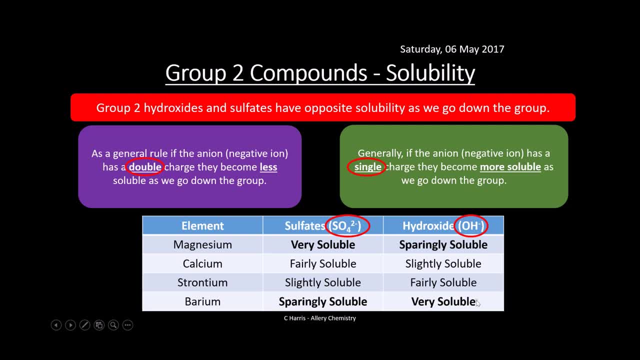 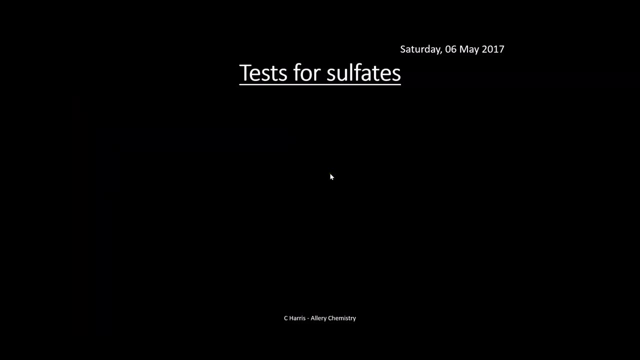 you can see here that magnesium hydroxide is pretty insoluble, but barium hydroxide is very soluble. so, as you can see, the solubility decreases. you've got to know about the solubility of these. that's pretty important, okay, uh right, okay, so test for sulfates using these solubilities. this: 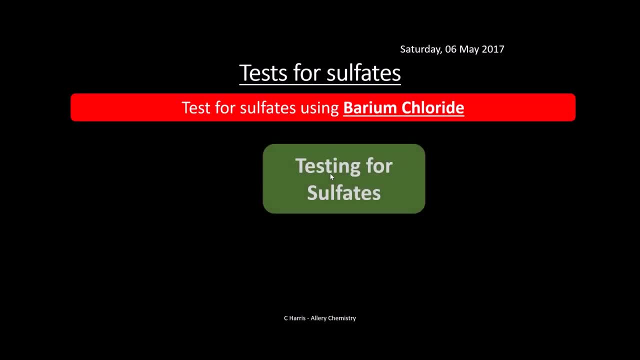 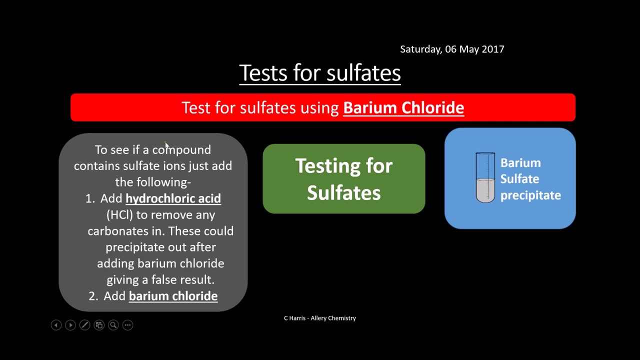 can be really useful. okay, so we test for sulfates using barium chloride. okay, so when we're testing for them, we're going to see if a compound contains sulfur ions. all we do is we do this following method: so we add hydrochloric acid first. basically, what this does is it removes or? 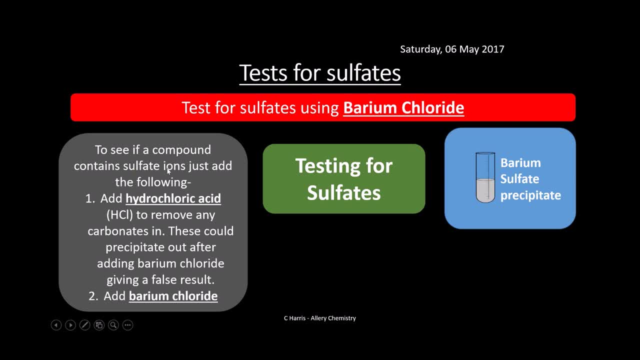 reacts with any carbonates that may be in there. um that um could effectively precipitate out when we add the barium chloride. um and this would give a false result, because we'd see a white precipitate, thinking that actually, yeah, we do have a sulfate in there and actually we don't, we just have a. 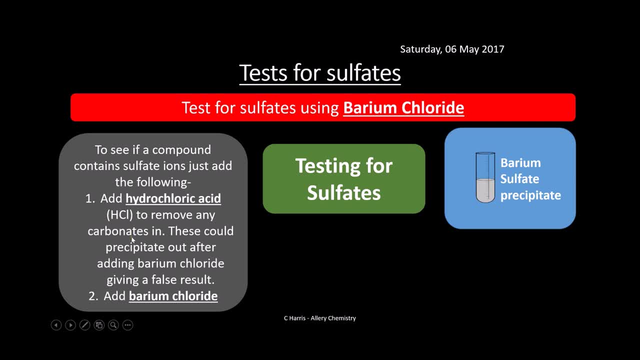 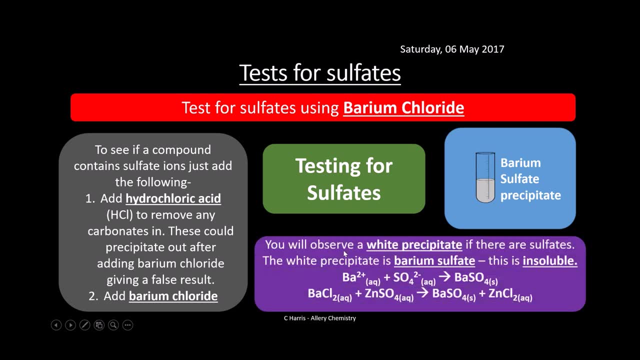 carbonate. so we basically remove this to mop up any carbonates left in there. it's naturally found. once we've done that, then we just add barium chloride um and you, surprisingly, and we get a white precipitate. well, not really. it's a bit of a joke. so 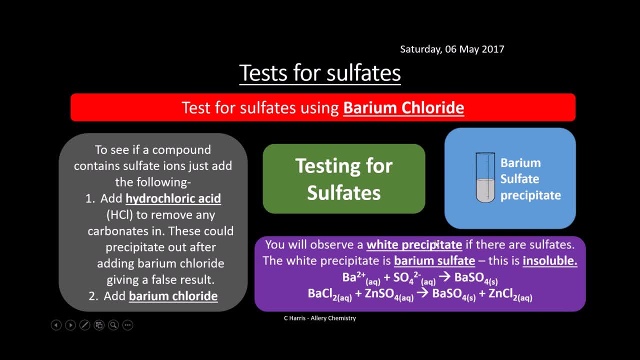 effectively. we do, yeah, we do get this white precipitate. there's no surprise really, because, uh, the reaction is barium chloride. reacting with, let's say, a sulfate, zinc sulfate forms barium sulfate, just in the previous slide. obviously we've seen that sulfates are insoluble. 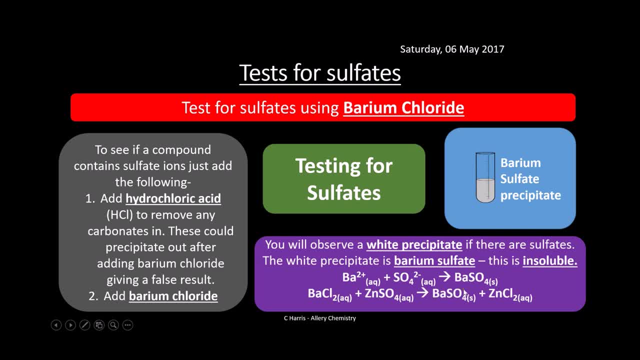 especially um. well, barium sulfate- sorry- is insoluble, so we're bound to get this white precipitate. uh, we get zinc chloride, which is obviously soluble. so we observe this white precipitate if there are sulfates. and this is because um you form barium sulfate, which is 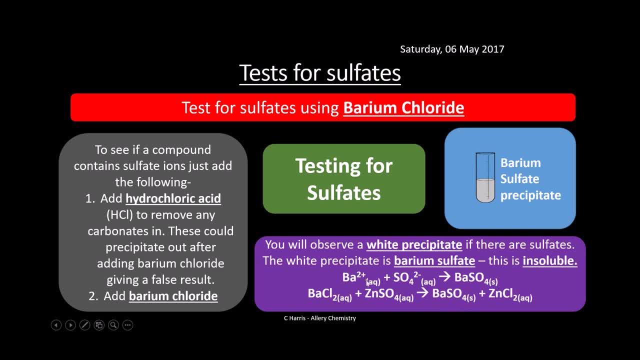 insoluble. the ionic equation is this: so barium ba2 plus reacting with sulfate so42 minus forms barium sulfate. notice the state symbols: aqueous, aqueous, solid. okay, we always form a precipitate. so if we see a white precipitate barium chloride, add that to your 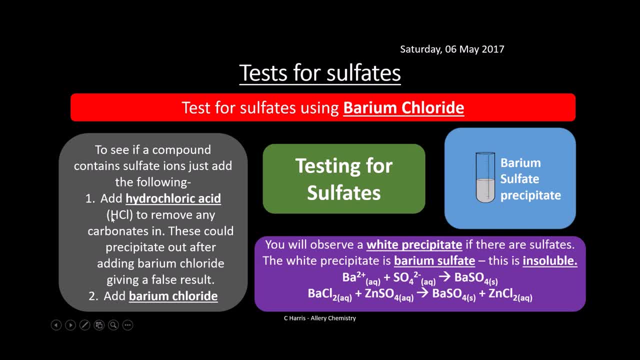 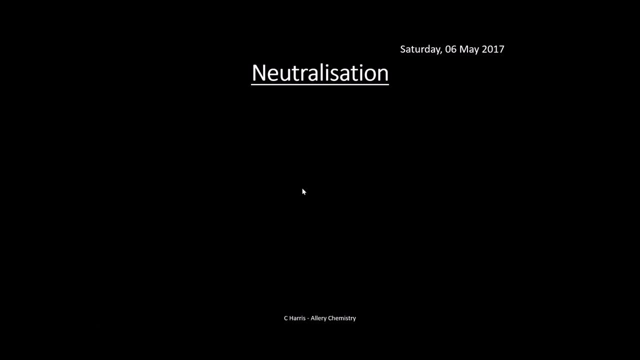 you compound. if you get a white precipitate, it contains a sulfate. remember to add the hcl to remove any carbonates. okay, neutralization. now these things are like we said and they can be used as alkalines and so group two compounds. they can be used to neutralize acids. so we looked at 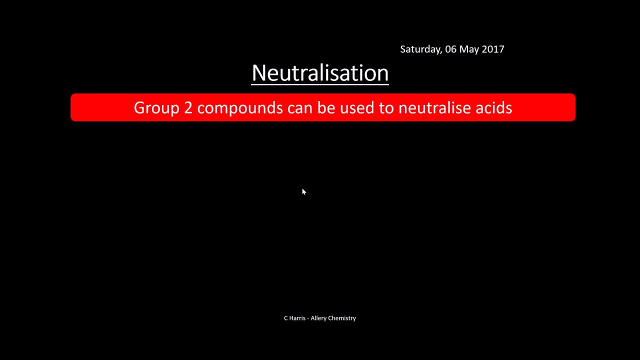 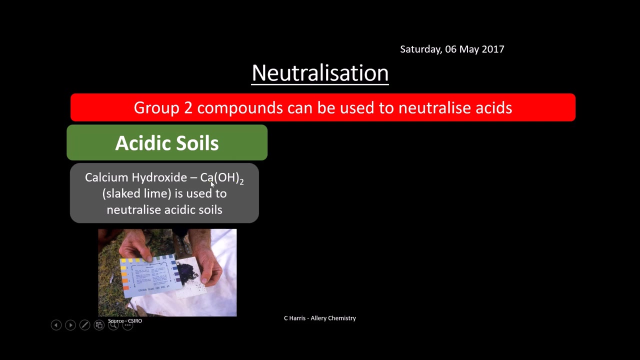 the one when we acted it with water and you formed your group- two hydroxides. they're alkaline, so we can use them to neutralize acids. so one example is with acidic soils, and so calcium hydroxide, um, which is caoh, is basically used to neutralize these soils, so we can spray this onto the soil. 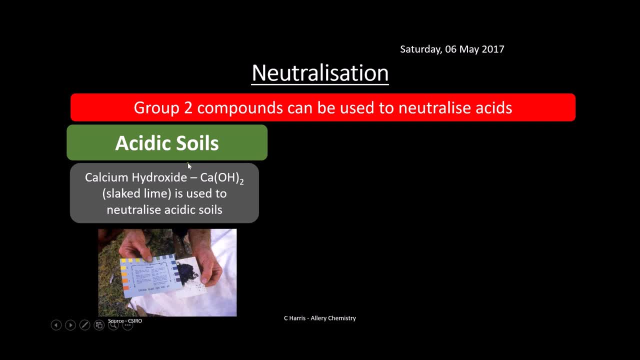 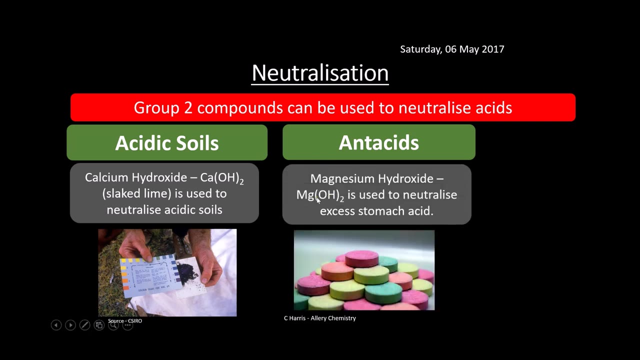 some plants prefer to um grow in less acidic soils. so if the soil is reasonably acidic, you spray some calcium hydroxide on and it just neutralizes the acidic soil. antacids: this is probably more common. again, we use magnesium hydroxide for antacids- m-a-m-g-o-h-2, and this is used to neutralize. 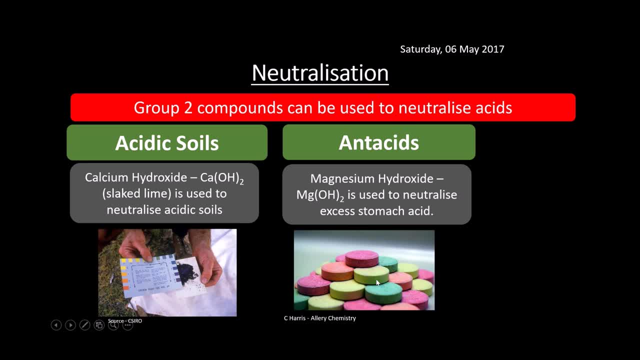 excess stomach acid. that may cause an acid to be neutralized so we can spray this onto the soil and obviously occur, particularly if you've eaten things like chilies. sometimes some people get a bit of excess acid, stomach acid buildup. you take magnesium hydroxide and it should settle. 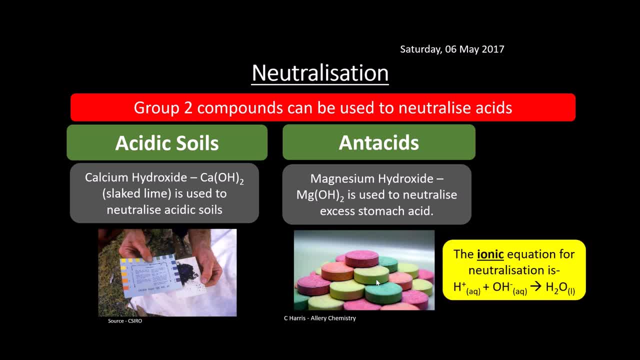 down neutralizes the acid. okay, so the ionic equation, dead easy. this one for neutralization: h plus, that's produced from the acid, oh, minus is from the alkaline that produces your neutral compound, h2o, which is a liquid. notice, your ions are always aqueous. okay, your water's liquid. 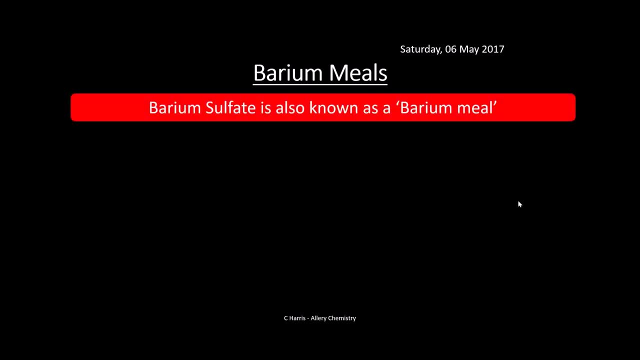 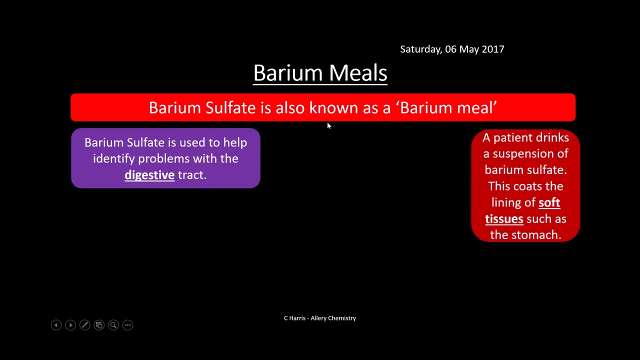 right barium meals, so these are pretty useful. uh, these used in medicine actually. so, um, the barium sulfate is also known as a barium meal. uh, barium sulfate is used to help identify problems with the digestive tract in particular. barium sulfate is pretty dense. actually it's pretty heavy pretty. 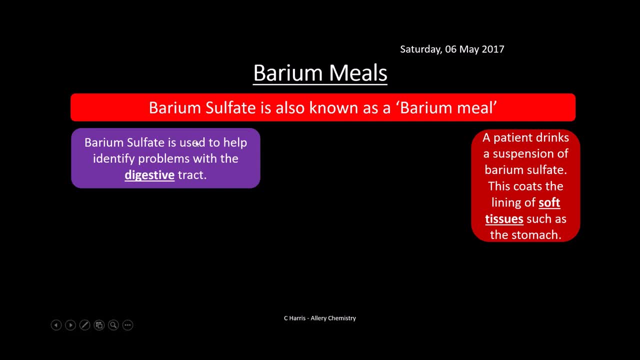 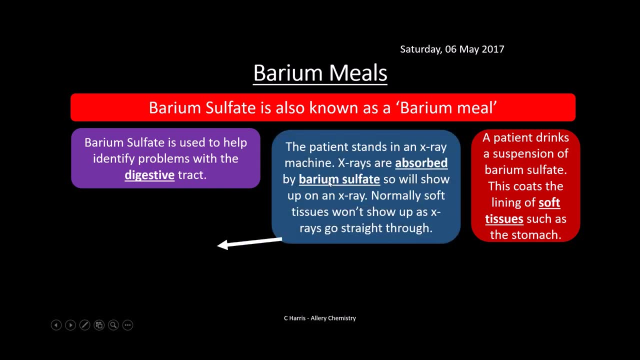 heavy material. so how it works: the patient drinks basically a suspension of barium sulfate and what this does? this lines the, the soft tissues within the body and basically the patient's hands in front of an x-ray machine. uh, and x-rays are absorbed by barium sulfate. you can see an. 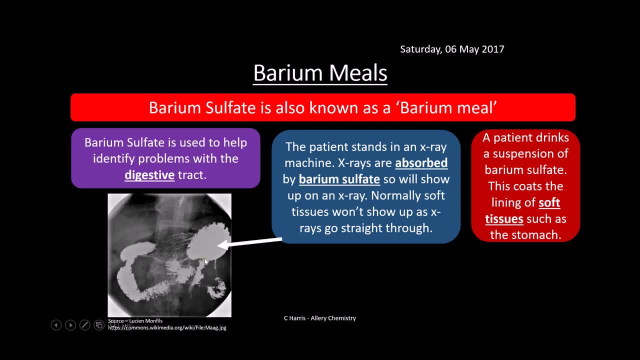 image here, um. so you can see that we've got some obviously white um dense areas. this is the barium sulfate inside the digestive tract, um and soft tissues. problem is that if we didn't use barium sulfate, all the x-rays would go straight through the soft tissue. so the barium sulfate basically. 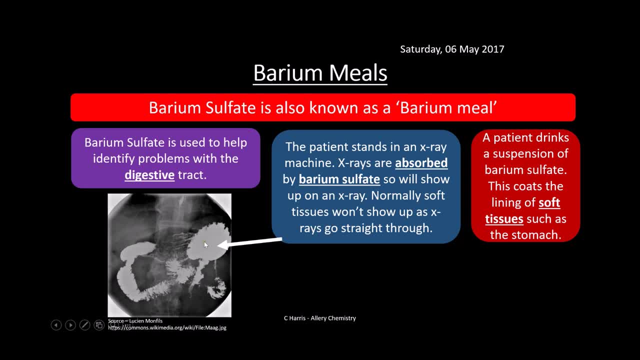 shows up parts of this now. I'm no doctor, so I don't really know what's going on here, but you could basically um look for things like blockages, things which aren't getting through the digestive tract, for example, so it's pretty, um, pretty useful for that thing. now, barium compounds are toxic, okay, so you've got to. 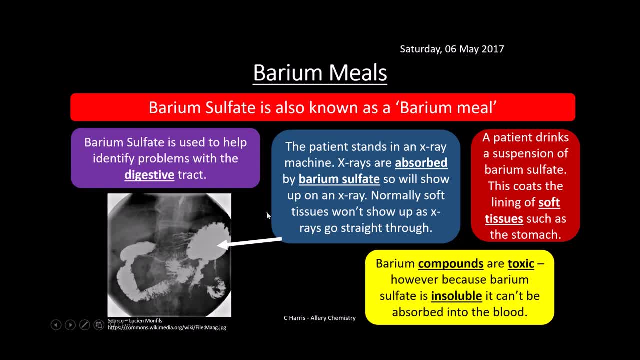 be really careful with this. yeah, we can ingest them, which seems a bit daft, but thankfully, as you know from the previous slides, that barium sulfate is insoluble, so it doesn't get absorbed into the blood, so that that's pretty useful. they ask this question: um, then you need to be able to. 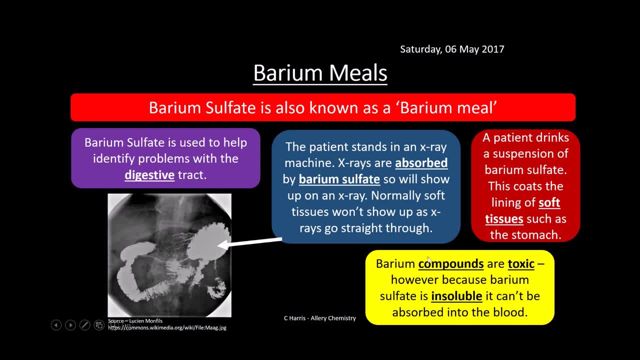 kind of refer to this and they might phrase it as toxic, and you might be sitting there thinking, well, that's quite bad, why? why would you take it? but just remember your solubility rules. okay, so we're just applying them- solubility rules- to a real life. 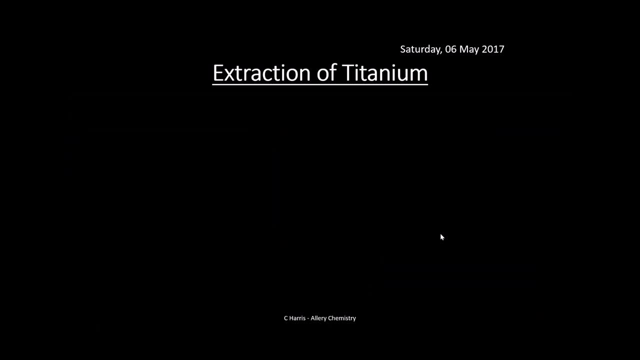 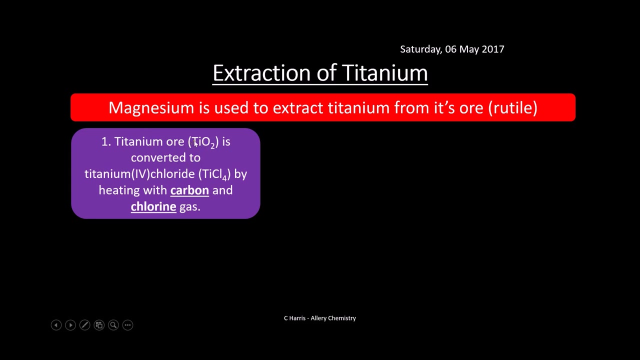 example. okay, extraction of titanium. now, titanium is one of these great metals. it's a lightweight metal but really tough and hard, so magnesium is used to extract titanium from its ore rutile. now magnesium is a grip to metal, um, so titanium ore is titanium dioxide, tio2, and it's converted to. 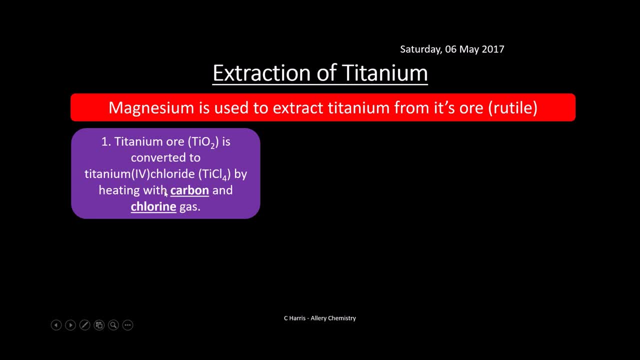 titanium chloride. titanium chloride first. all we do with that is we just heat it with carbon and chlorine gas. now we've got to heat it with chlorine because what we don't want is the carbon reacting with the titanium, because it forms titanium carbide, which is brittle and that pretty 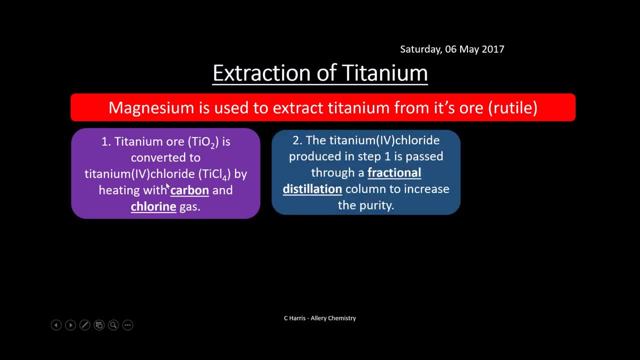 much ruins your, your reaction. so we react it with chlorine, so we form the ticl4. then, once we form the ticl4, we then basically pass it through a fractional distillation column. we increase the purity so we get rid of any other bits that might be in there, like titanium dioxide and carbon etc. so we just 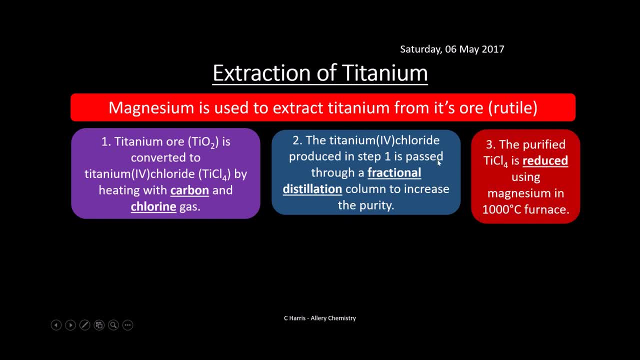 try and get a pure sample. then the purified titanium um titanium chloride tetrachloride is reduced. we use magnesium to do this uh in a 1000 degree celsius furnace. we're using really high temperature but want to remove the chlorine from from titanium uh in this compound to get pure. 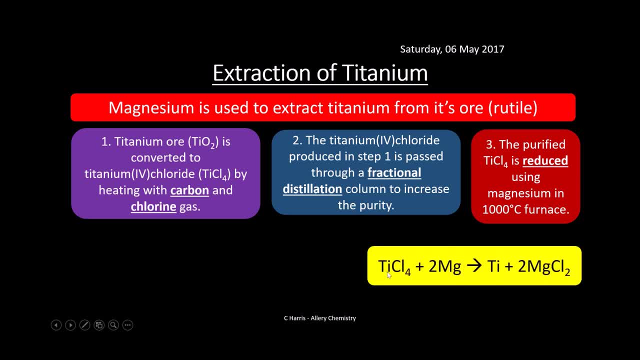 titanium. so we're using magnesium and here's the reaction to ccl4. we're acting with magnesium. we get pure titanium and magnesium chloride okay, so this is why we can use it so effectively. we're reducing it. so remember, titanium here is plus four. titanium here is zero because it's an element. so that's reduction. so the magnesium is reducing the. 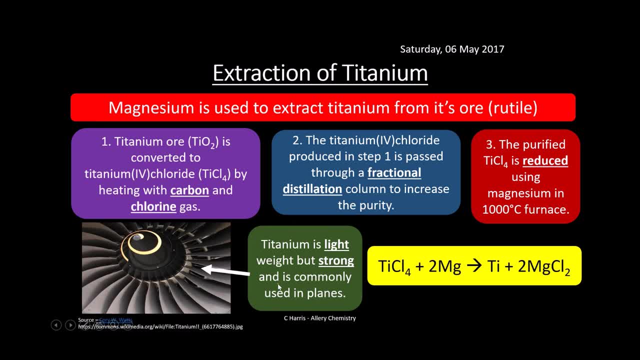 titanium chloride: uh, lightweight, like i say, very strong, commonly used in planes. you can see the fins of this jet engine: uh, that basically allows it to um be uh used in the kind of uses because you don't want heavy metals in a plane, you want the plane to fly um, so yeah. 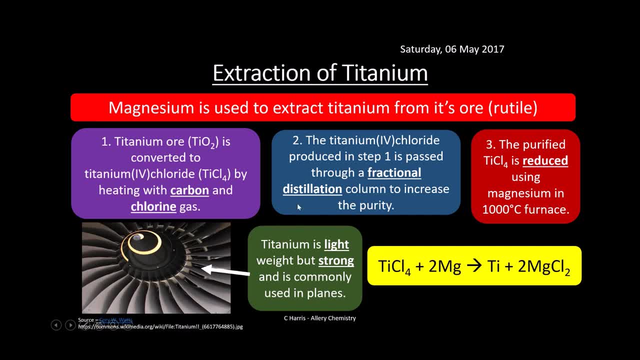 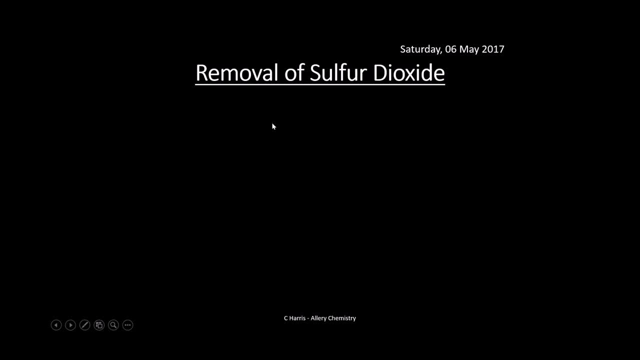 okay, so that's the type of thing we're looking for for extraction of titanium. okay, uh, removal of sulfur dioxide. so, like i say, um, these things are alkaline, so they're really good in terms of reacting with acids. okay, so a particular use for this is, um, using calcium. 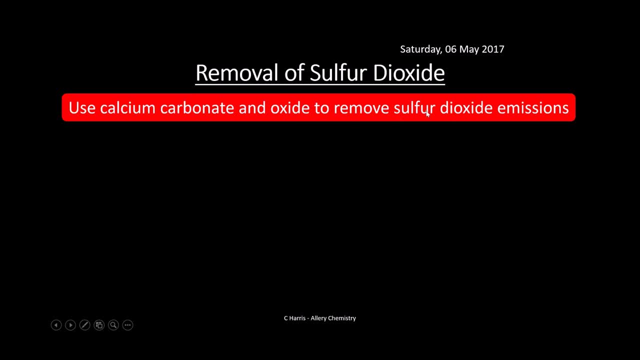 carbonate and oxide um, so both to remove sulfur dioxide emissions. so this is normally produced. when you burn things like fossil fuels in power stations etc. you produce sulfur dioxide as a byproduct. isn't good, you don't want that getting into the atmosphere. so yeah, like i say, we can. 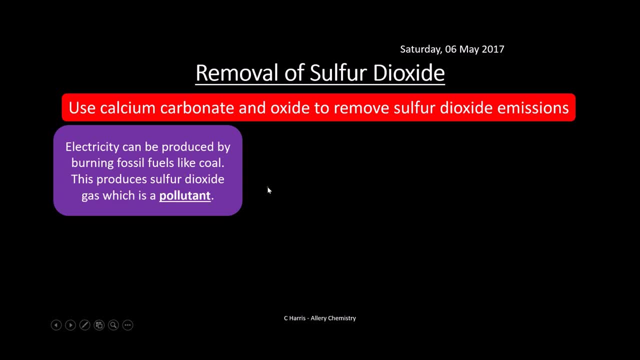 produce electricity burning fossil fuels, it produces this harmful pollutant. so what we use? we use something called wet scrubbing and this is a method where, effectively, we um neutralize the acidic gases coming from the burning of fossil fuels. uh, it's an acid. it's acid causes acid. 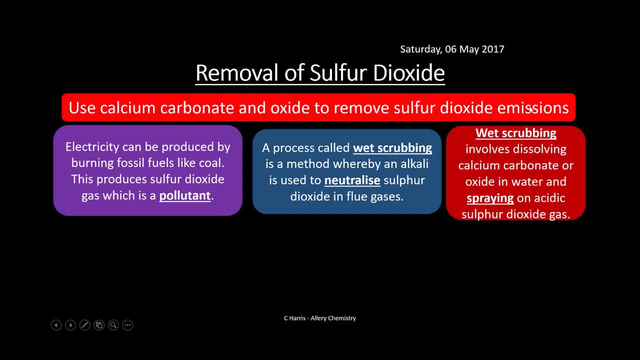 rain this if it gets into the atmosphere, so you don't really want it in there. you so wet scrubbing. basically, what we do is we spray this um this solution of calcium carbonate or an oxide either, or we spray it onto the sulfur dioxide gas as it leaves the? um chimney and